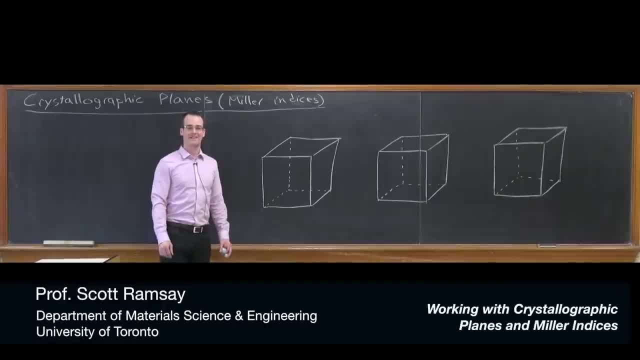 Hi, Let's take a look at determining crystallographic planes, and we're going to use a set of numbers similar to what's done in directions, except we call them Miller indices and they're determined differently, obviously because they're describing a plane. So the process is going to start. 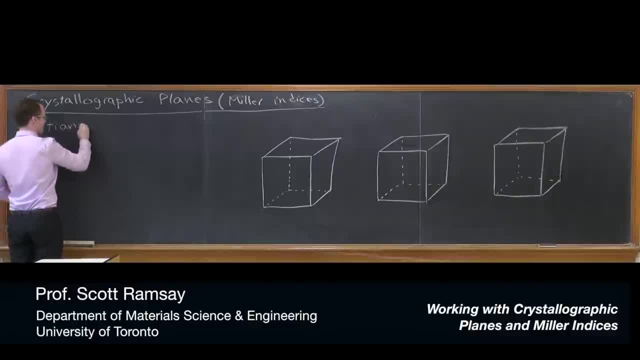 by remembering that you can translate a plane if necessary, and it doesn't change the plane, as long as it's parallel to the original. That's what translation implies: We're translating it parallel to the original, But we have to do this step if the plane crosses through. 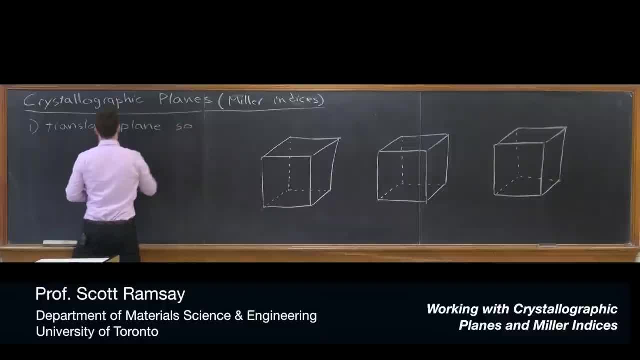 our origin Translate plane. So origin Origin Is not on the plane. Of course, another way of stating that same fact is: you can define a new origin. You can define a new origin. that's not on the plane. The origin is your. 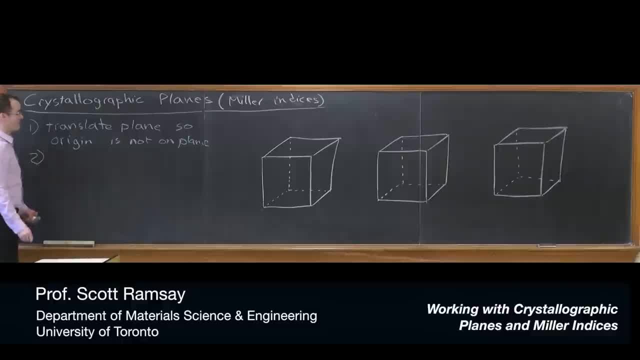 tool to work with, to use to make your life easier. So once we've done that, then we can determine distance to intercept plane by traveling along each axis, along each axis from the origin, and then, in this step, you have to realize that you may have infinity introduced. 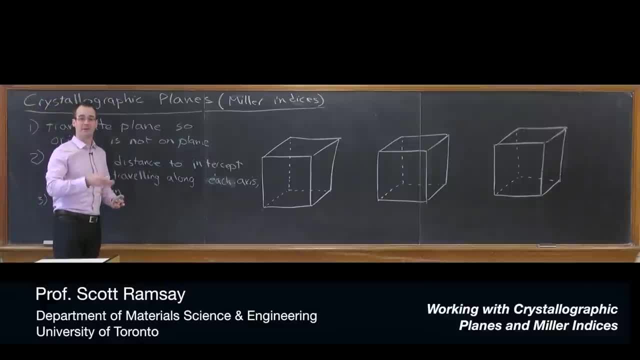 if the plane is parallel to one of the axes, you could travel infinitely far along that axis and never intercept the plane. so we've got infinity in there. we're kind of funny people in material science. we like to keep notation in a very specific way, and fractions: we don't like fractions. 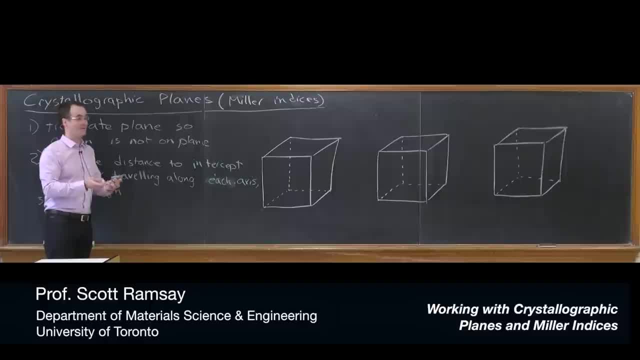 you don't know that from directions and infinity? signs are pesky, they use up a lot of space. we'd rather express it as zero. how do you make infinity into zero? take the reciprocal. so we take the reciprocal each and every time, and even if there's no infinity in the particular plane, 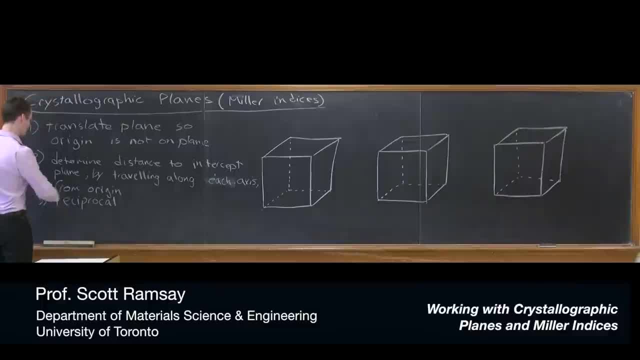 that you're working with, you still take the reciprocal to be consistent. so you take the reciprocal and then we enclose in parentheses, and then we enclose, and often we just use the placeholder letters h, k and l to refer to general Miller indices for a plane. 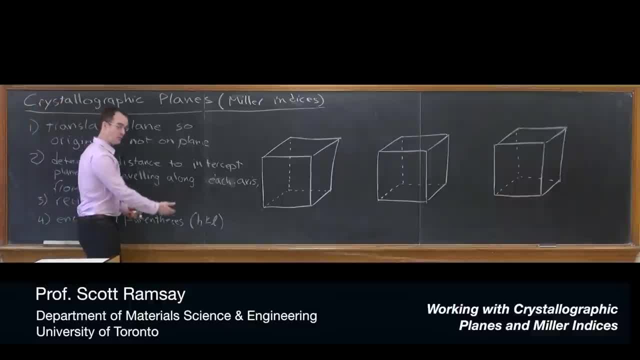 if there's any negative signs, we move them over the top, like what we do for directions, and I'll write that down. just to be complete, negatives go above and no commas. no commas, alright, good. so let's take a look at a plane. let's take a look at my all-time favorite plane. 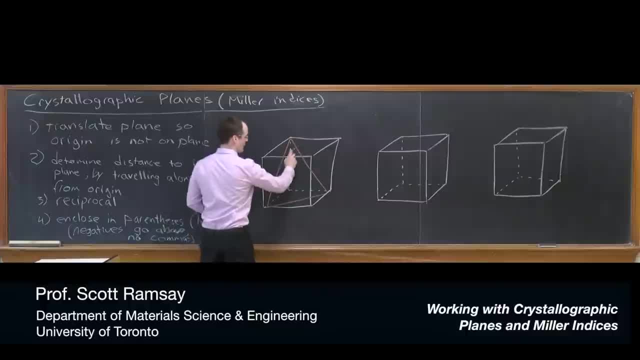 this plane here cuts off the back bottom left corner of the plane and cuts off the center of the cube, so we can actually, in this case, start with this conventional origin as our origin. so what we're going to do is- I'm going to proceed through in this same order here- 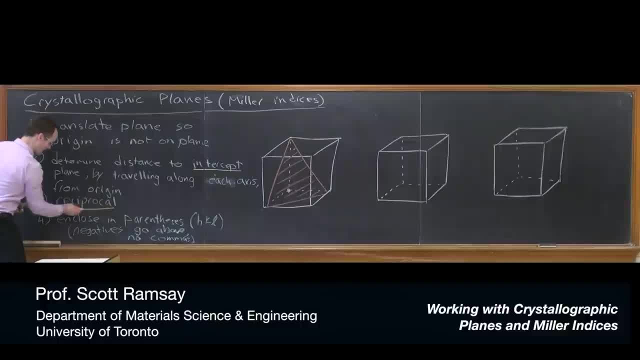 I'm going to determine the intercept, I'm going to take the reciprocal and then I'm going to enclose. so we're going to do that. we're going to determine the intercept, take the reciprocal and then we're going to enclose for x, y and z. 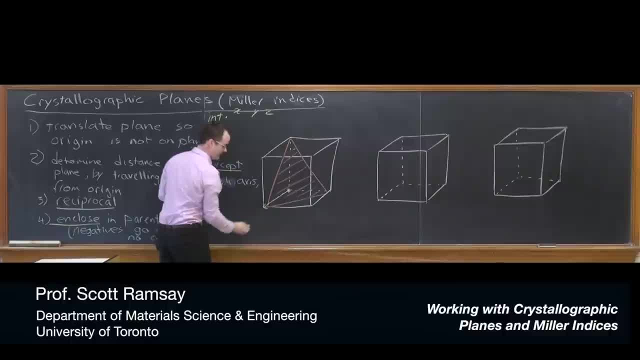 so from this origin here we travel 1 in the x direction. we would travel from that origin 1 in the y direction to hit the plane. and from this origin here we would travel 1 in the z direction and hit the plane. there's no reductions necessary. 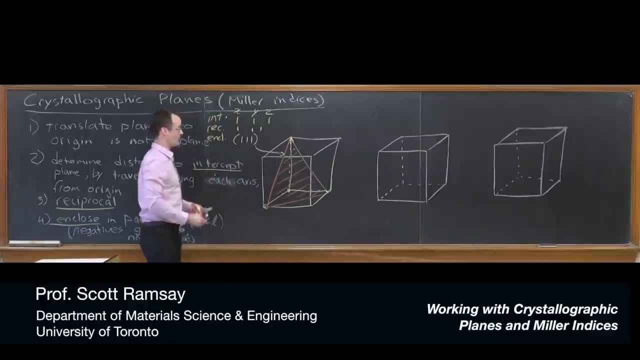 and the enclosure then becomes 1, 1, 1. this is the 1, 1, 1 plane. what about if we take a look at another another plane over here, perhaps? perhaps this plane right here? alright, so this plane crosses through the y axis at half. 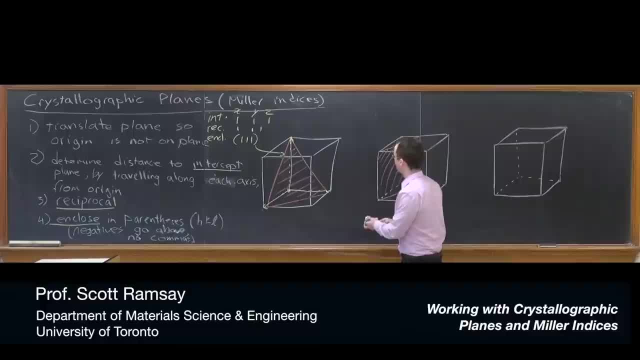 of the lattice parameter in the y direction. so again, we're going to go systematically. I mean, there are shortcuts you can take, but let's do it systematically. at first, intercept: reciprocal enclosure. I actually missed a step and that would be reduction and it's going to be important on this step here. 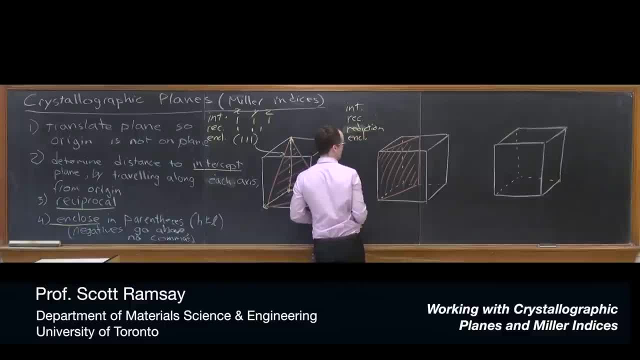 reduction and then enclosure. so again we can start with this conventional origin. we would travel 1 in the x direction, y and z. we would travel a half lattice parameter in the y, one half, and how far would we travel to z? well, it's actually parallel to z. 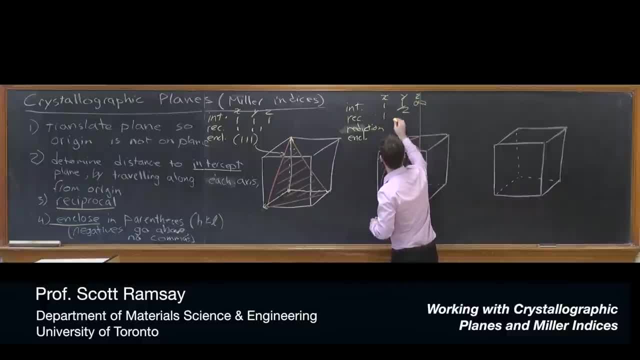 so we would travel infinitely far. so our reciprocal gives us 1 to 0. the reciprocal is taking care of the reduction. actually, sorry, I should have thought of that so we didn't need to do that extra reduction step. if we had needed to, we would have cleared the fraction. 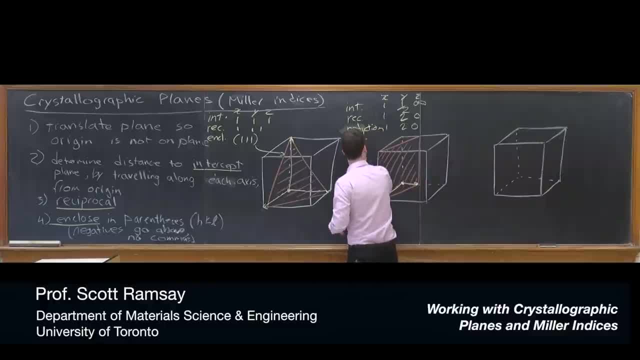 just by multiplying across by the lowest common denominator, and so the enclosure then becomes 1 to 0. that's the 1 to 0 plane. finally, we could look at families of planes, and these are planes that look the same in two dimensions. they've got the same atoms in the same positions. 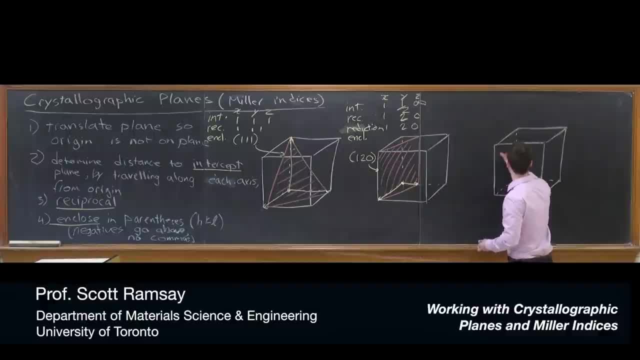 they would have the same linear packing fraction. so, for example, you know the faces of a cube well. the faces of the cube are: this front face is the 0 and the back face is the direction. it's the 1, 0, 0. you can see the 0s in the x.